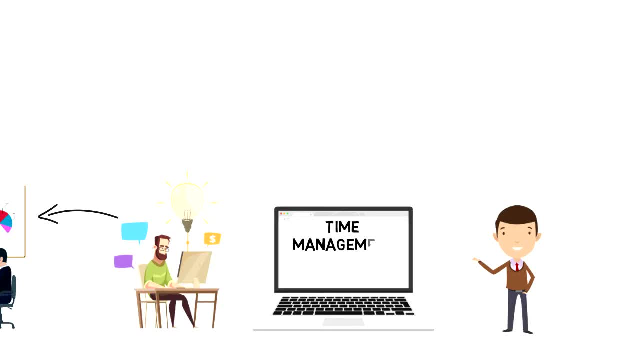 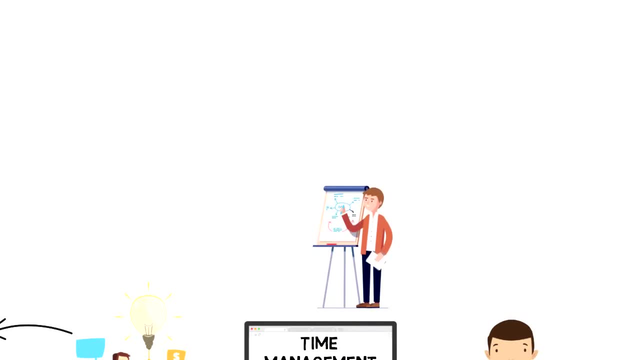 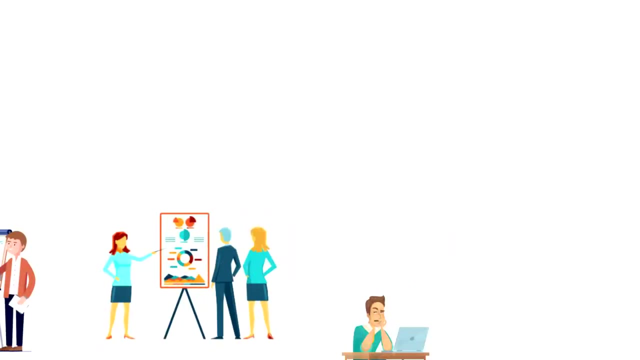 and hit the bell icon to get updates on my latest videos about time management and productivity. Prototype is an early sample, model or release of a product built to test a concept or process. If you are creating or building something new, then it might be quite an expensive process that. 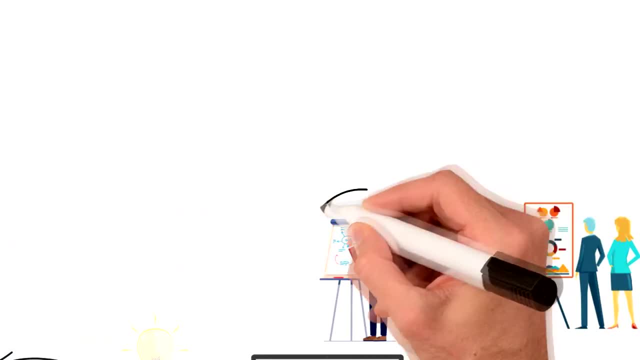 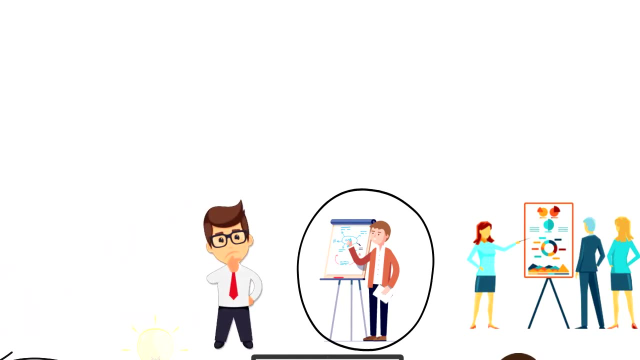 might end up not working as intended. So the solution is to create a prototype for a much cheaper cost to see if it's worth building the full version of the product. For example, when I was developing my second mobile game, me and my team came up with 10 different 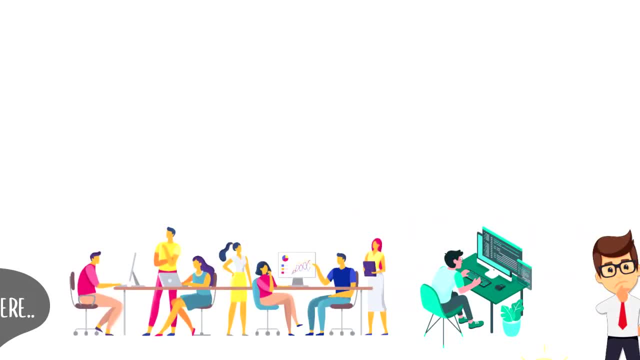 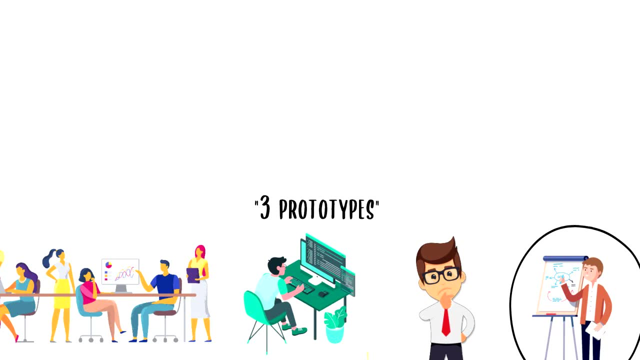 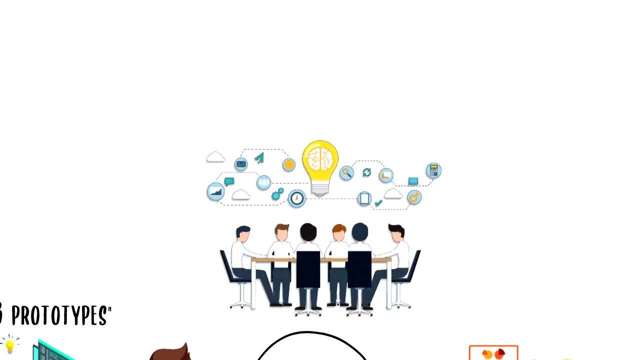 ideas for a hypercasual mobile game. Then we evaluated and decided to create three prototypes to see what they would feel like on a mobile device before making a decision about what game to develop. This enabled my team to get a real feel about different game concepts and therefore 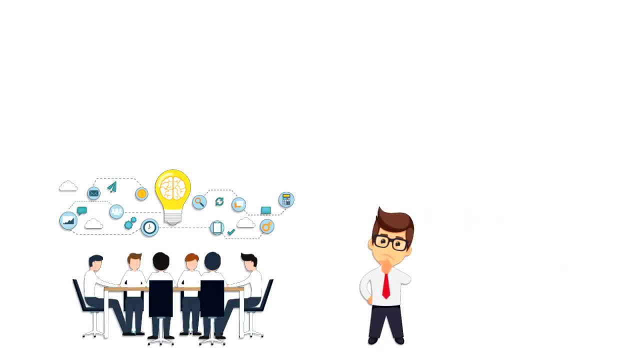 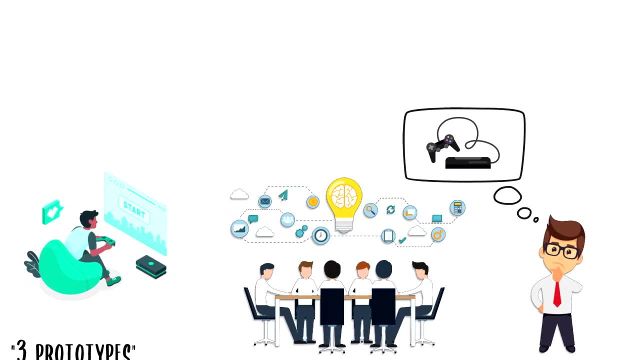 make more informed decision. Of course, it is important to note that the prototype is very minimalistic version of what the real end product will look like. Therefore, only key features can be tested, while you have to imagine how everything else will sit around the core concept. I think that prototypes are a great tool that can be used to test new 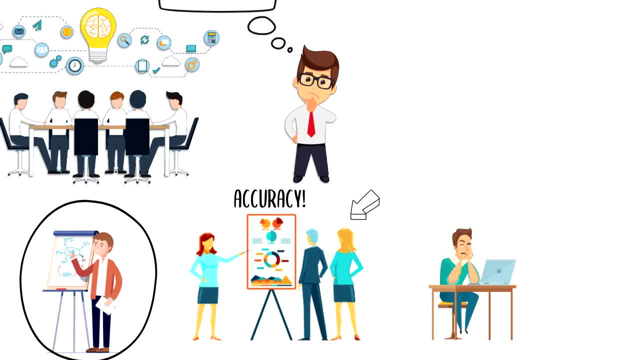 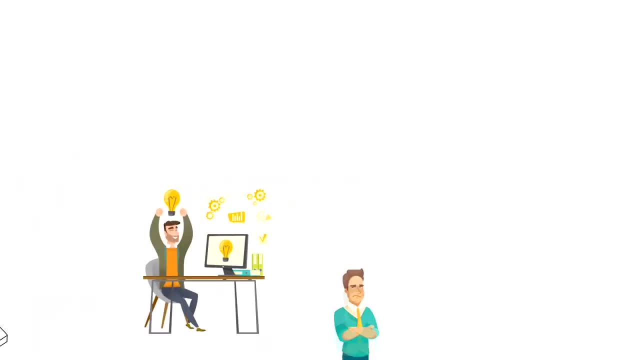 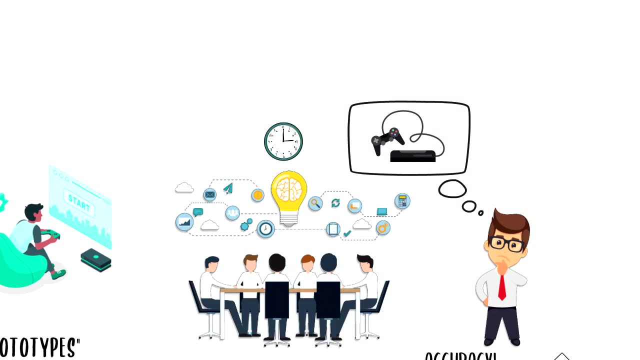 concepts and ideas with quite a high accuracy. When we come up with new ideas, they often sound great in our heads, but when we try to bring them to reality, it doesn't always work that well. So building a prototype can potentially save you a lot of time and money when it comes to developing. new products or products that you want to develop in the future. If you want to build a prototype, you will need a lot of time and money. but if you want to build a prototype, you will need a lot of time and money. but if you want to build a prototype, you will need a lot of time and money when it comes. 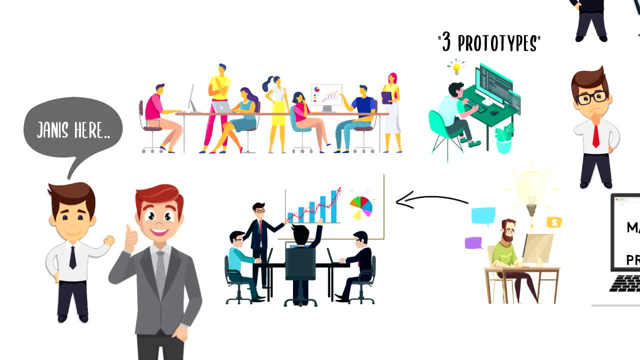 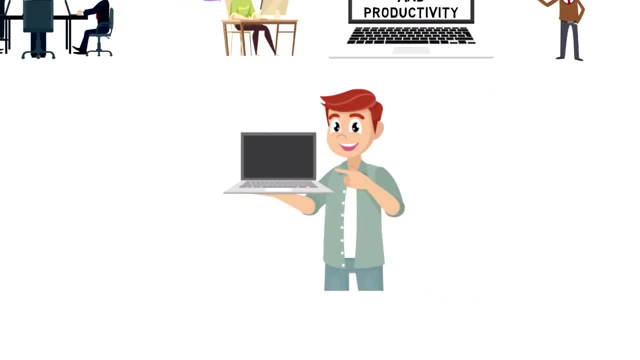 to developing new products or services. I hope that you enjoyed this video and I was able to give you a quick summary of what a prototype is and how to use them. If you enjoyed this video, I would really appreciate if you could press the like button, as this will help the video reach more. people and spread the message.